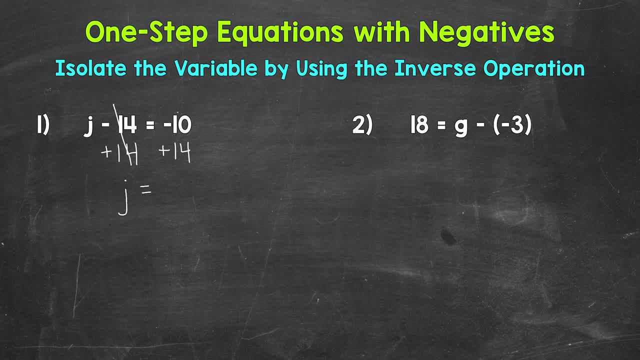 negative 10 plus 14.. We are starting at negative 10 and increasing in value by 14. So we end up with positive 4.. j equals 4.. Now, one thing I do want to mention. we always have the option to come. to the side in order to show work or setup. So let's do that. So let's add 14 to the right side of the equation and then on the left side of the equation, we have negative 10 plus 14.. So we end up. 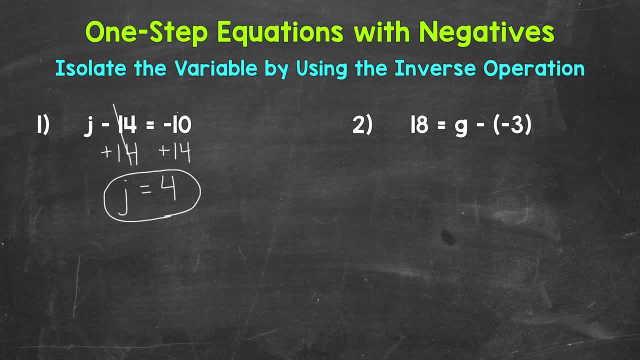 a problem differently. For example, negative 10 plus 14, we solved vertically, so up and down. If you prefer to work through that horizontally, you can always rewrite the problem off to the side. So negative 10 plus 14, that equals 4.. So you always have that option. Now j equals 4.. That's our. 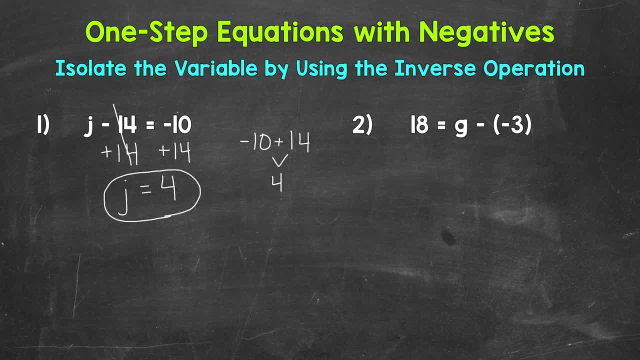 solution. We can always check a solution and make sure that we have the right solution. So let's plug 4 in for j and see if this works. So 4 minus 14 equals negative 10.. 4 minus 14 does equal. 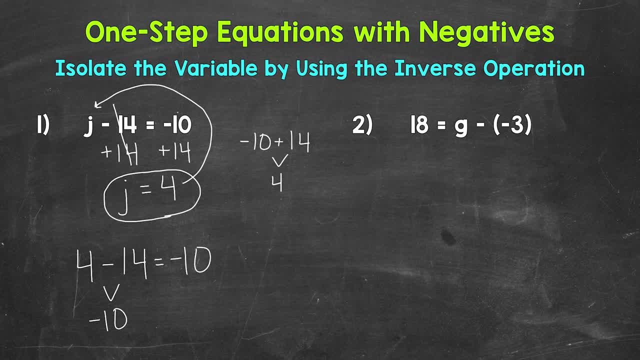 negative 10.. So we have the correct solution: j equals 4.. Let's move on to number 2,, where we have 18 equals j equals 4.. So we have the correct solution: j equals 4.. Let's move on to number 2,. 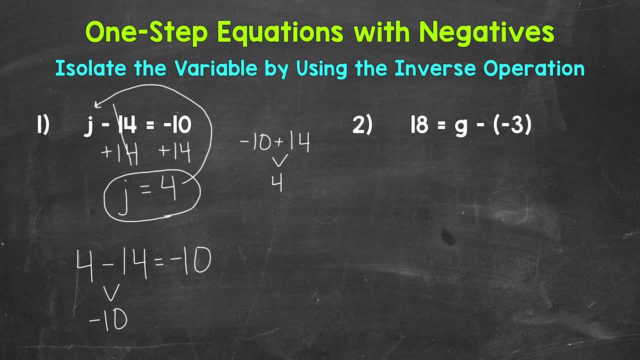 g minus negative 3.. We need to isolate that variable of g. Negative 3 is being subtracted from g. We need to undo that subtraction by using the inverse operation. The inverse of subtraction is addition. So let's add negative 3 to the right side of the equation. 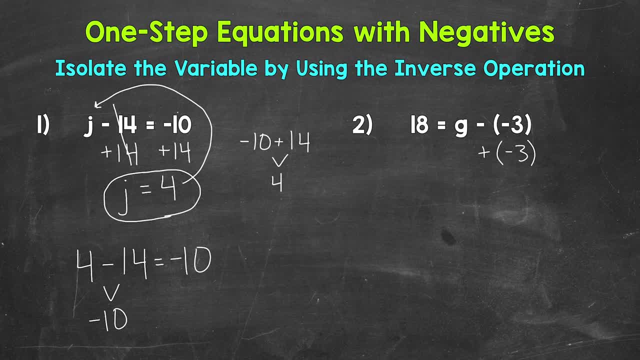 Whatever we do to one side, we must do to the other. So let's add negative 3 to the left side as well. Let's take a look at the right side of the equation Now. when we subtract a negative, we are actually increasing in value. 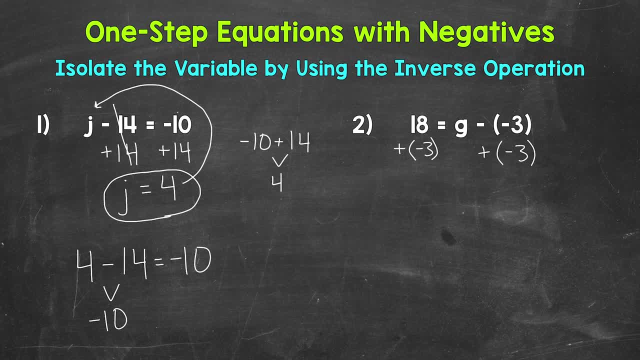 So we are increasing g's value by 3. So by adding negative 3 to that side of the equation, these cancel out and equal 0. So our variable of g is So: g equals. And then on the left side of the equation, 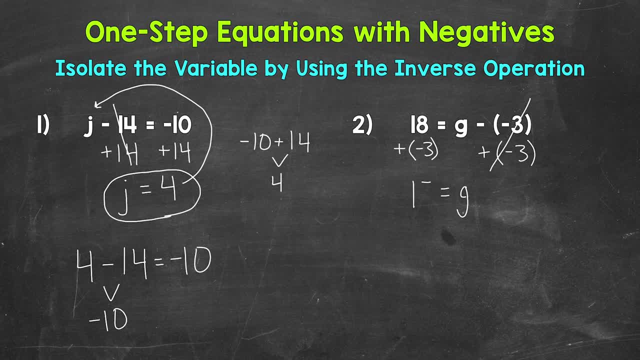 18 plus negative 3 equals 15.. So g equals 15. And we can rewrite that with the variable coming first. Now, if we look back up at the right side of the equation, that can be a little confusing to think through, because it looks like we have. 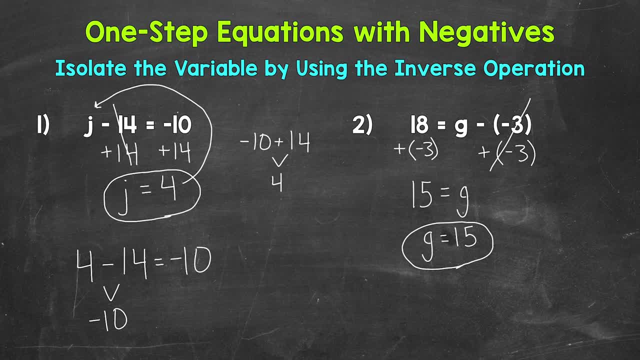 negative 3 plus negative 3,, which would equal negative 6. Not that 0, which isolated our variable. But keep in mind, when we subtract a negative we increase in value. So g is increasing in value by 3.. 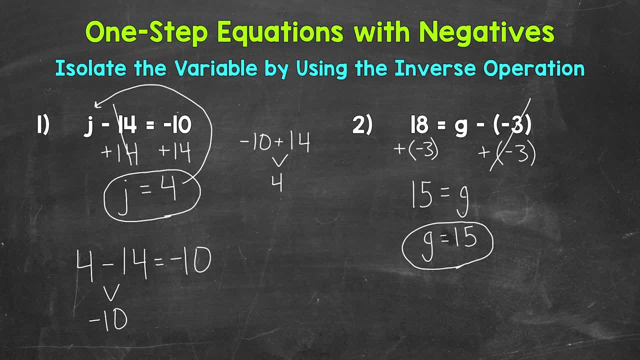 By adding a negative 3 to that side of the equation, we are canceling that increase out to equal 0. And our variable was isolated. Here is an easier way to think about it: Whenever we subtract a negative, we can think of this as adding a positive. 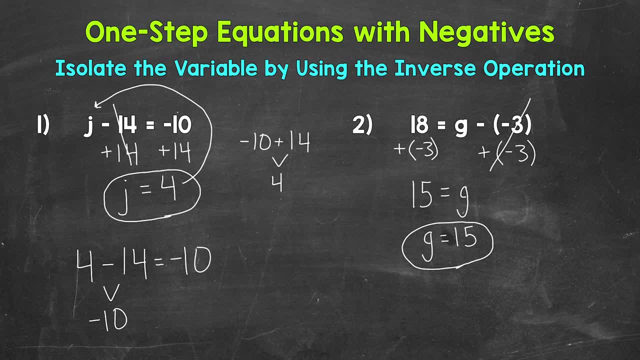 And remember, when subtracting we can always add the opposite. So this works out. We can actually rewrite this as: 18 equals g plus 3.. g plus a positive 3. Because again we can add the opposite. So add and then the opposite of negative 3 is positive 3.. 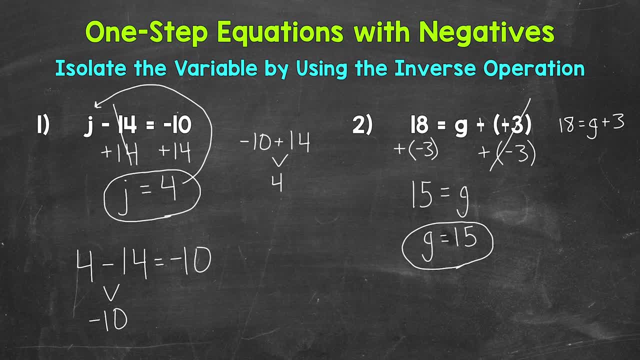 So you can always rewrite the equation if you're subtracting a negative to add a positive. Let's go through the rewritten equation and see if we still get 15.. We need to isolate g. 3 is being added to g, So let's undo that addition by using the inverse operation. 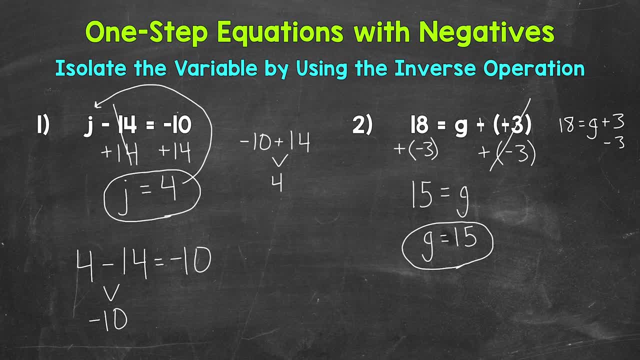 which is subtraction. Let's subtract 3 from the right side of the equation. Whatever we do to one side, we must do to the other. So subtract 3 from the left side as well. On the right side, we are adding 3 and subtracting 3..